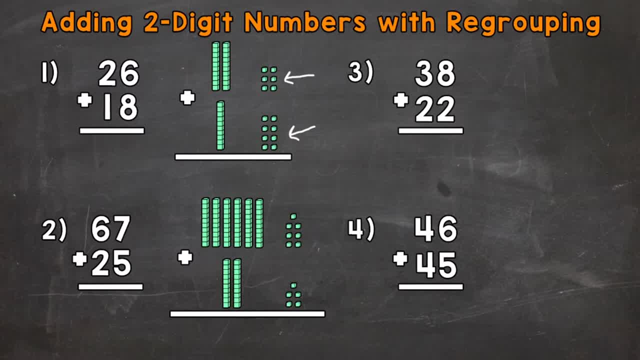 ones place. We can't fit a two-digit number into the ones place, So what we're going to do is make a group of 10 out of the ones and regroup or carry it over to the tens place. So we have six ones. 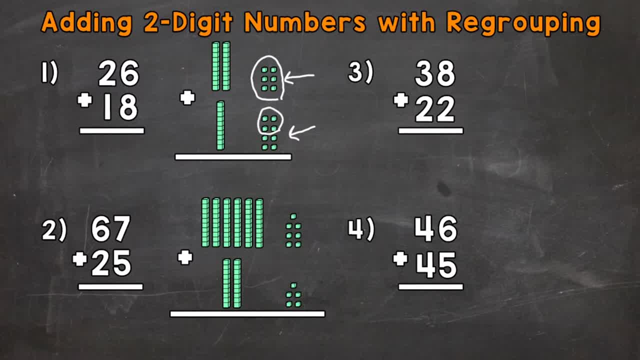 plus another four ones would give us a group of 10.. So we're going to regroup that group of 10 over to the tens place And I'll put a stack there representing a group of 10.. So we have four ones left in the ones place. So we'll put that four in the ones. Now we count how many tens. 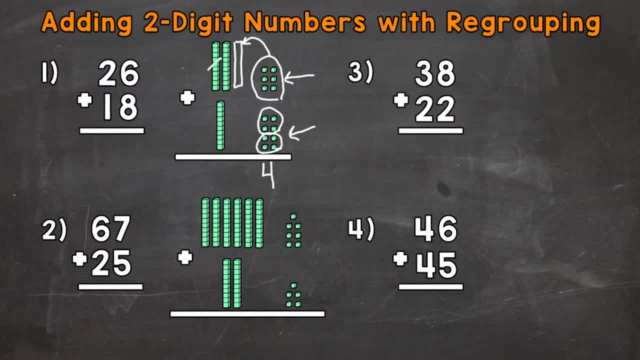 we have. So we have one group of 10, two, three and four, So four tens. So our answer is 44. Let's solve that to the left without the base 10 blocks as well, and see if we get the same thing. So six plus eight again is 14.. 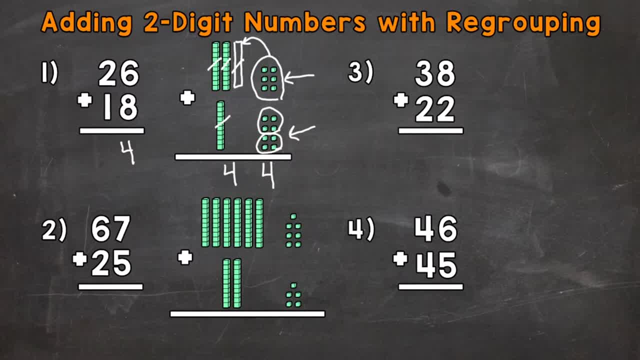 So we'll put the four in the ones place and then regroup the one group of 10 from 14.. Now we're going to sum the ones with the tens place. Now let's add the tens: One tens plus two tens plus one tens. So one plus two is three plus one is four. So we get 44 again. 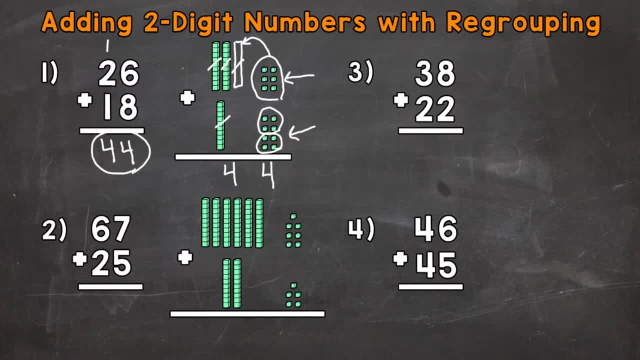 44 is our final answer Now. the four in the tens place represents four groups of 10 and has a value of 40.. The four in the ones place represents four groups of 10 and has a value of 40.. The four in the ones is 2016.. Now, more tens. in the tens place The four, two tens At number 1.. Now that picture here what I did, Kleiner, let me put that over here. The four number is 10.. So spring it right from number 1.. 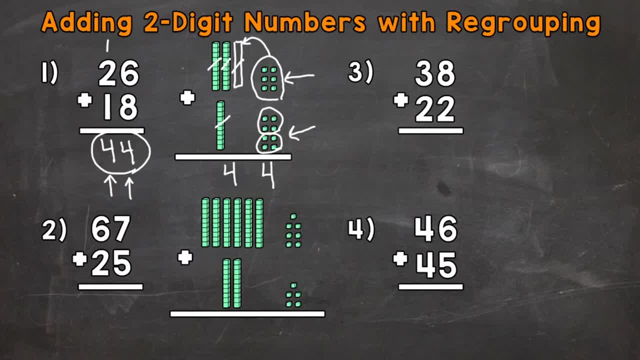 represents four ones and has a value of four. Let's do another one and move on to number two, where we have 67 plus 25.. And remember, always start with the ones. So 7 plus 5 is 12.. Now we can't fit a two-digit number in the ones place, so we're going to need to regroup. So seven ones. 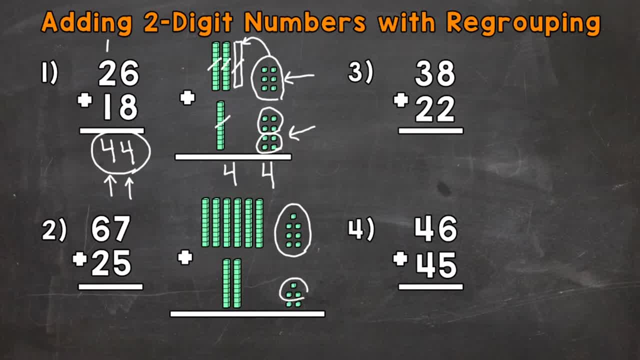 plus three ones gives us a group of 10 that we can regroup to the tens place. So let's regroup, bring that over to the tens and we're left with two ones right here. So we have a two in the ones place. Now we count how many tens we have: One, two, three, four, five, six. 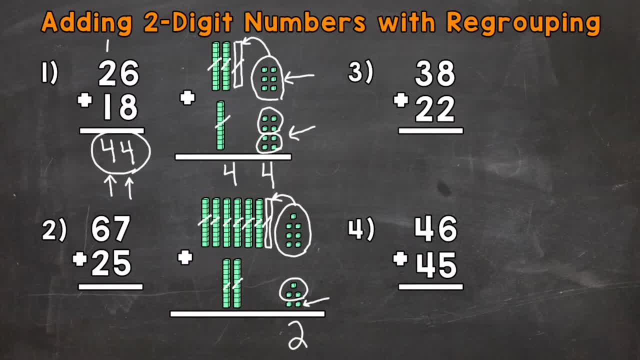 seven, eight and nine, Nine tens. So we get an answer of 92.. Let's do it without the base 10 blocks. So 7 plus 5 is 12.. So we put the two in the ones place and regroup the one group of 10. 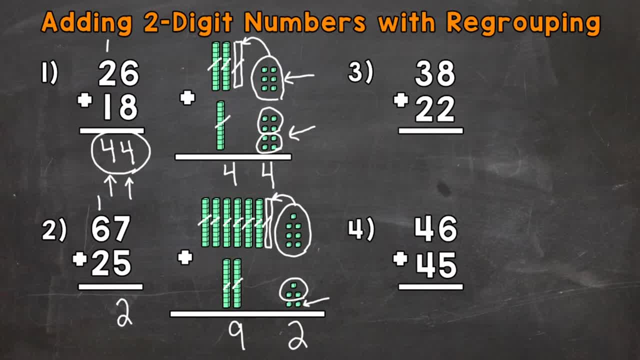 from 12 in the tens place. So now we have one 10 plus six tens plus two tens. One plus six tens plus two tens plus three tens. So now we have a group of 10 plus four tens And we regroup the one group of 10 from 12 in the tens place. So now we have one 10 plus six tens plus two. 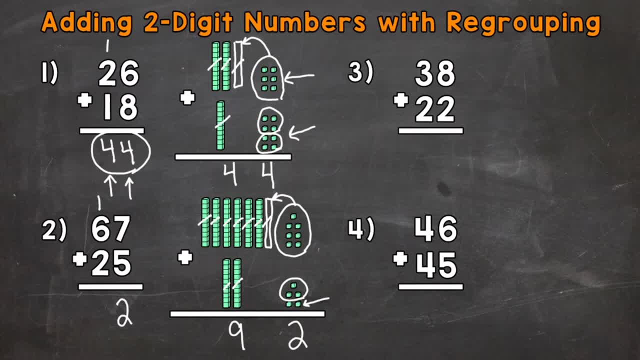 six is seven tens plus two tens is nine tens. Now that nine has a value of 90 because it's in the tens place and the two has a value of two because it's in the ones place. Now, another way to think of this: the tens. let's take a look at the tens place. We have one ten which has a value. 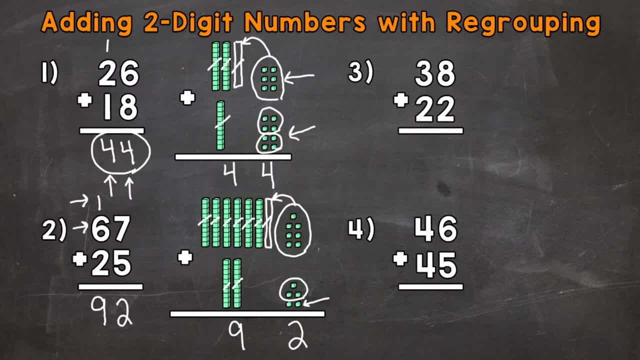 of 10, plus six tens, which has a value of 60, plus two tens, which has a value of 20.. So 10 plus 60 plus 20 is 90. And that nine has a value of 90,, like we talked about, because it's in the tens. 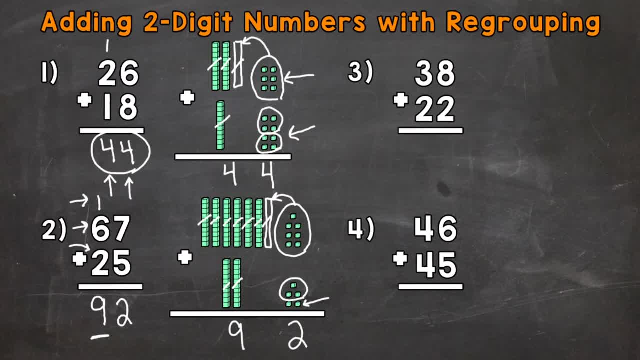 place. So think about the value of the digits you're adding due to the place that they're in as you're going through the process Understanding these values. that's important to understanding what's going on within these addition problems and math in general. So again, 92, our final answer. Let's move on to numbers. 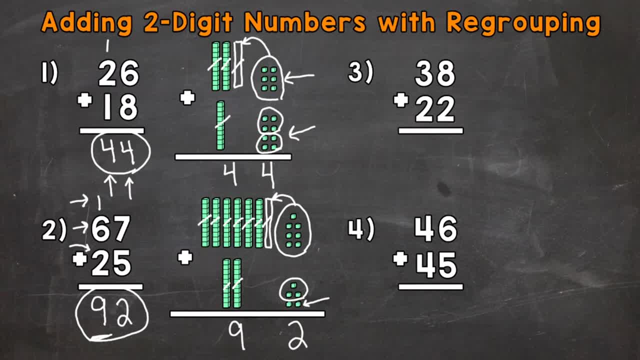 three and four. And in these problems we're not going to use base 10 blocks. We'll start with number three, where we have 38 plus 22.. Start with the ones. So eight plus two, That gives us 10.. So one group of 10.. So we put our zero here And like numbers one and two. 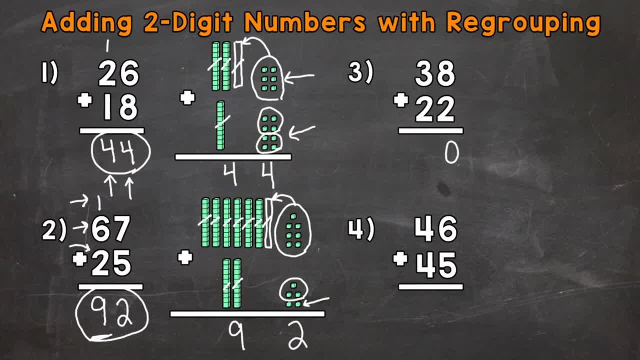 we can't fit two digits into one place, So we need to regroup our one from the 10, our one group of 10 with the tens. So now we add our tens, So one, 10 plus three, tens plus two, tens, One plus three. 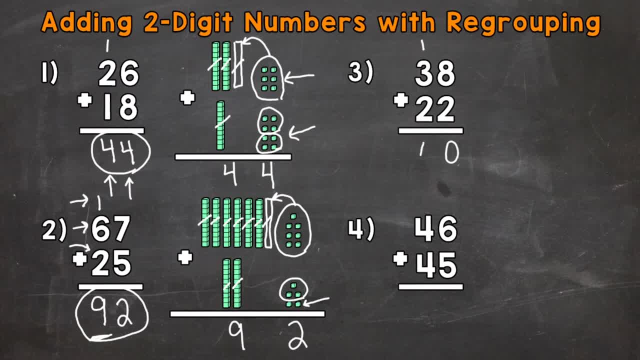 is four plus two is six, So we get a final answer of 60.. Now to recap there. as far as the tens place, one 10 has a value of 10.. Three tens has a value of 30. And two tens has a value of 20.. 10 plus 30 is 40,. 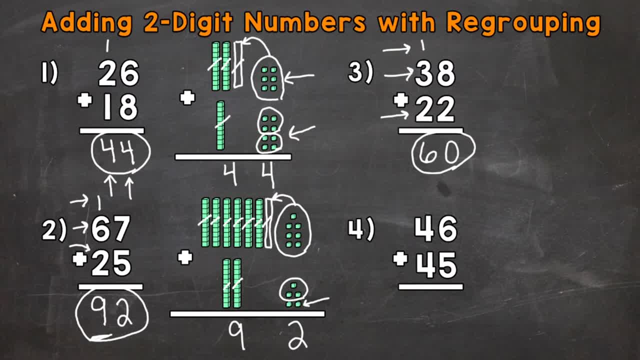 plus 20 is 60.. So that aligns with our answer. We have a six in the tens place that has a value of 60.. Let's move on to number four, where we have 46 plus 45.. Start with the ones. So we have six plus. 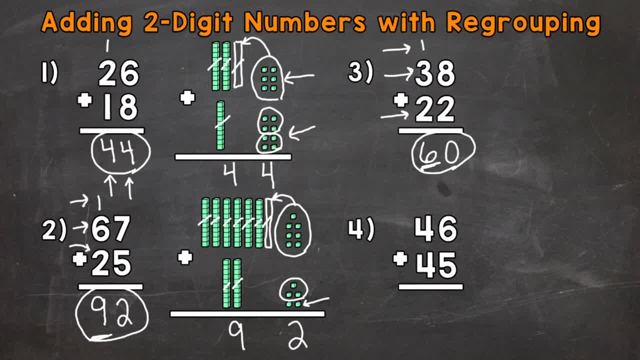 five, which is 11.. So we put the one from the ones place in 11 in the ones place and we regroup or carry the one group of 10 to the tens place. Now we have one 10 plus four tens plus four tens. 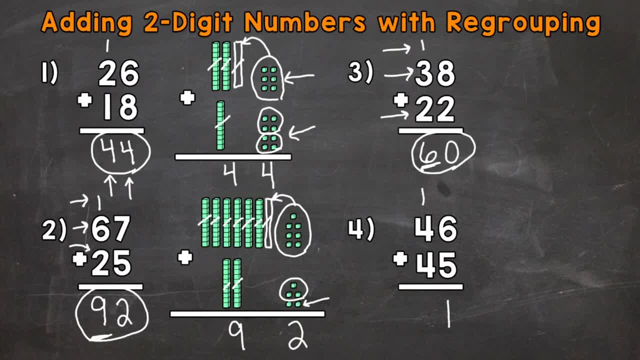 or 10 plus 40. So one plus four is five plus four gives us nine. So we have a nine in the tens place. Now that nine has a value of 90, because it's in the tens place, And then the one in the ones place has a. 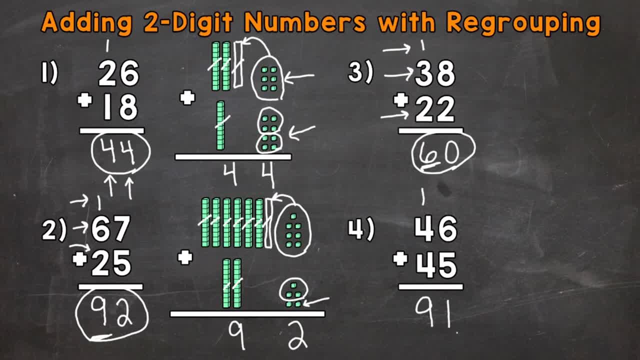 value of one because it's in the ones place. So a final answer of 91.. So there you have it. There's how you add two digit numbers with regrouping. I hope that helped. Thanks so much for watching. Until next time, Peace.